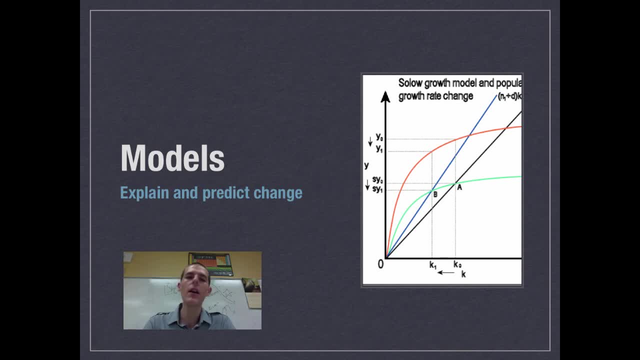 of models. we think of things that we can touch and see and feel and manipulate, But models aren't always physical. A lot of models used in science are actually graphical models, like you got there on the right. So what scientists will do is they'll take their data, they'll run it through. 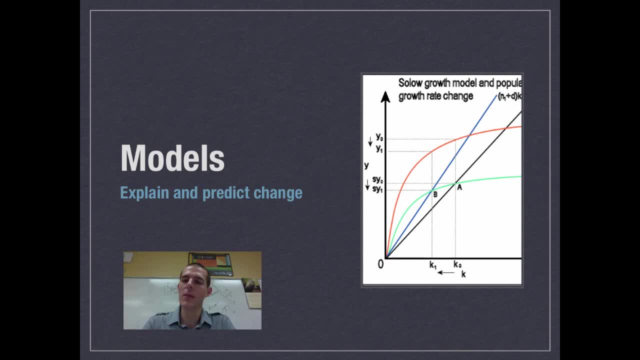 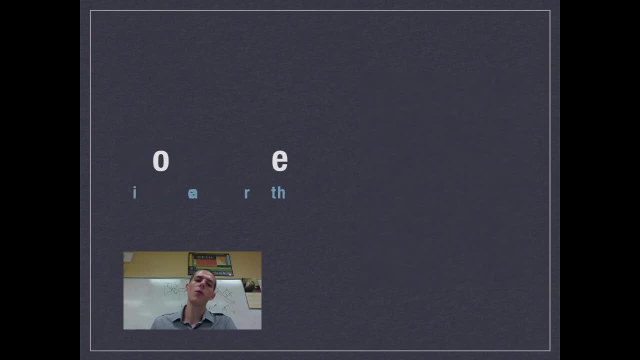 some formulas, they will graph it out and that is their model. that's going to help them to predict what is going on in a situation And throughout the rest of this video we're going to be talking about population growth models. But before we get into talking about those models, you need to know. 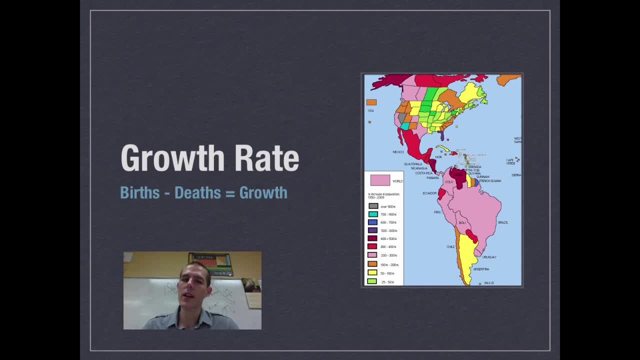 how to do some calculations. First, one is just a simple growth rate calculation, and this is easy. It's just asking you: how much has your population grown or shrunk? Births minus deaths equals growth. So that one is the easy calculation, The one that's more. 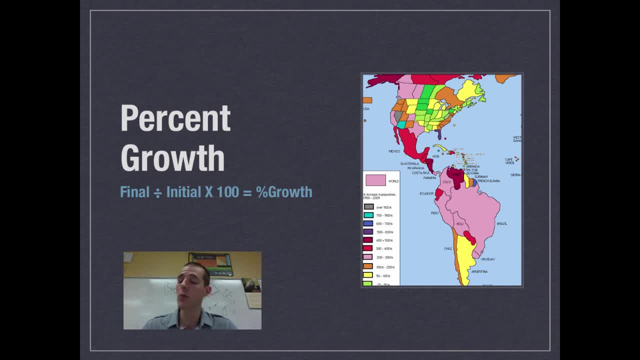 complicated, and the one that you'll probably see more frequently in apes is a percent growth calculation, And this is asking you to calculate what percent is the population growing or shrinking, usually every year, or something like that, And it's an easy calculation to do. All you got to do. 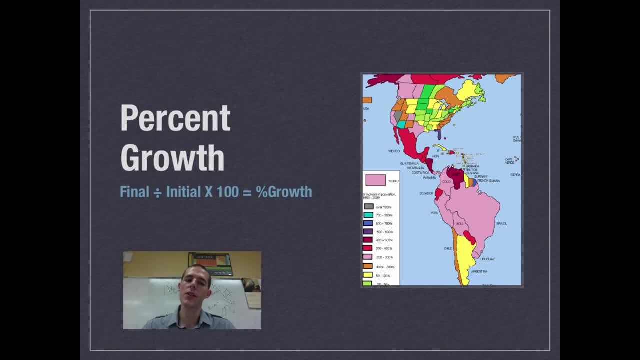 is: take your final population divided by your initial population and multiply that by 100. So a couple of things to be aware of when you're doing this. Let's say that your final population is 1,500 people. Your initial population was a thousand people. If you do this division, you get 1.5. 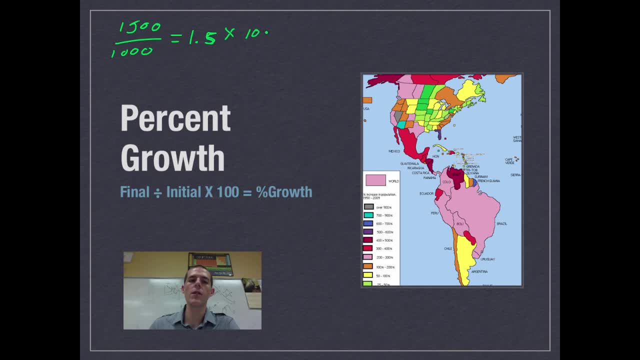 as your number and multiply that by 100, and that's going to tell you that your population is now 150% of the original. Now, this doesn't mean that your population has grown by 150%. It means that has grown by 50% because if you had the same population, that would be 100%. so you have. 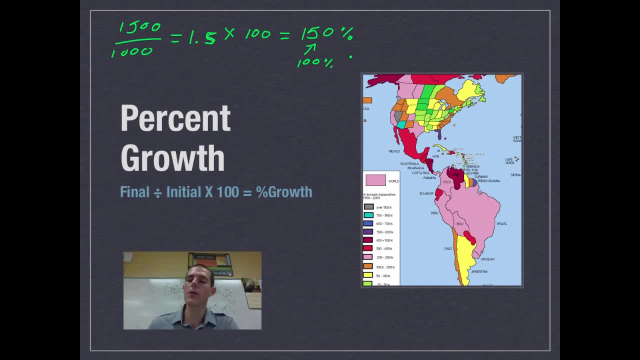 added 50% to your population, so that would be 50% positive growth. If let's say you had 500 as your final population, 1,000 as your initial, obviously that's going to be equal to one half, which is equal to 50%. so in this case your population has shrunk, you've gone from. 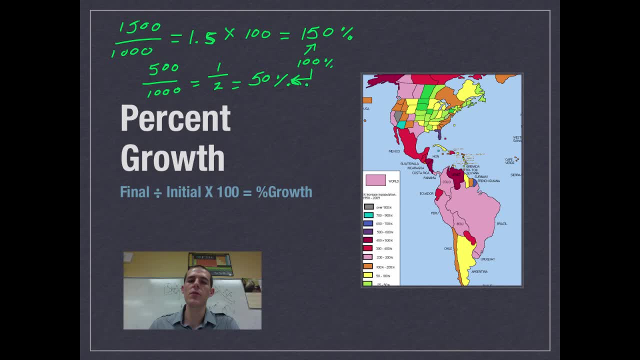 100% to 50%, which means that you have lost 50% of your population. so when you do these percent growth calculations, make sure that you be aware of whether your number is bigger than 100% or smaller than 100%. that's going to tell you whether your population has grown or shrunk. 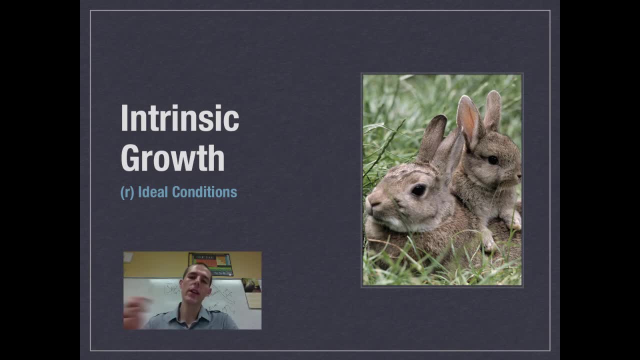 Next thing to be aware of is intrinsic growth. Now, intrinsic growth is a number that you have to consider. If you have a percent growth calculation, you want to the absolute maximum number of babies that an organism can have, without any limits at all. it is denoted by the letter R, lowercase art. to be specific, 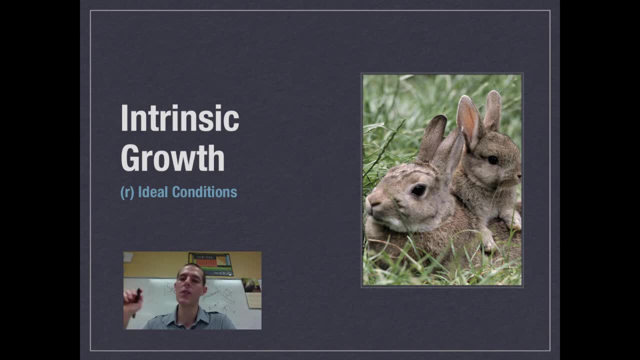 and, like I said, this reproduction under ideal connect conditions. so you give an organism no predators, maximum food, completely perfect conditions. how many babies can they have? in every animal on earth? every plant, every living organism has got a natural intrinsic growth rate. for humans you can see that our 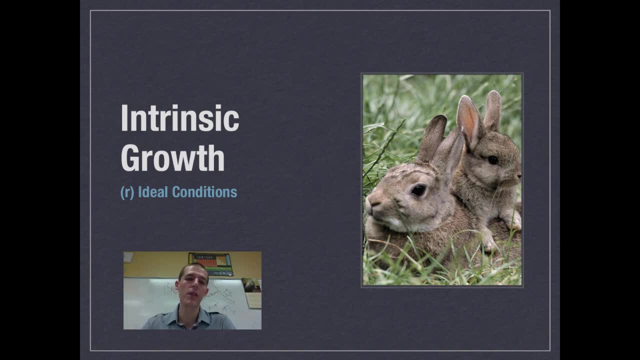 intrinsic growth rate is probably about one per nine months, because a woman can have a baby every nine months. technically we'll call it maybe ten months, but that would be our intrinsic growth rate. something so like rabbits, you know, you always hear the term reproducing like rabbits. rabbits can. 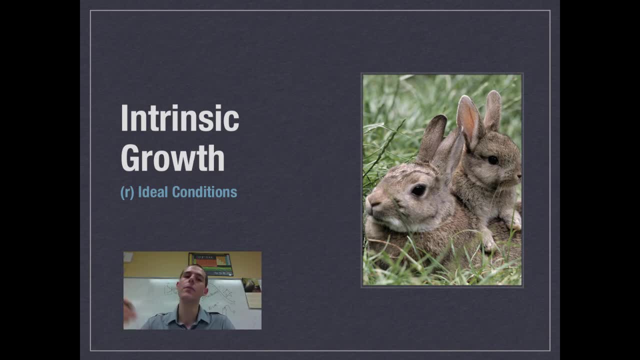 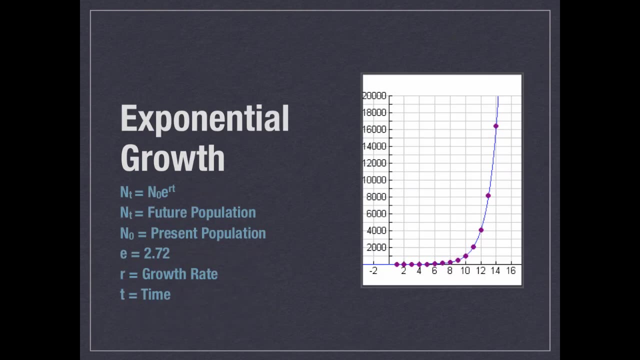 have a ton of babies multiple times during the year, so their intrinsic growth rate is much higher than the intrinsic growth rate of humans, which leads to this idea of exponential growth. now you a couple things to know about exponential growth. there is a huge formula for calculating it. the biggest thing you need to be able to do is you. 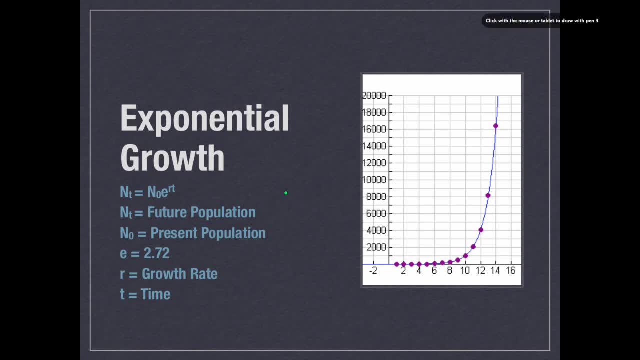 need to recognize an exponential growth graph, which is this guy right here. this is what you get. if an organism is allowed to grow all the way up to its intrinsic growth rate, there is nothing stopping it. there is no environmental pressure, no predation. it just grows like mad. so you see that population is growth. 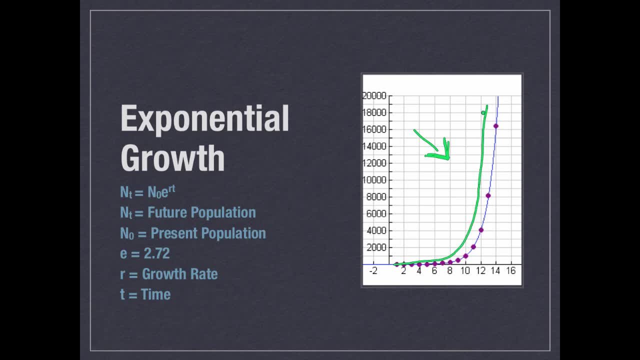 is slow, slow, slow and then it takes off all at once is what we're seeing in the human population right now. to calculate exponential growth, there is a formula right here: in sub T is equal to in sub zero ERT, and here's what each of these terms mean. so if you get a question like this, you can plug things. 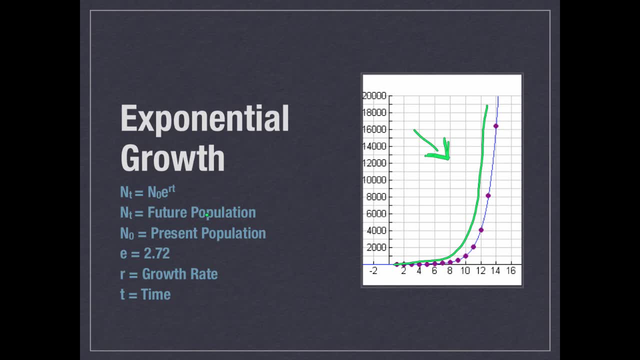 in in sub T is the future population. so what we are doing in this formula right here is we are calculating a future population size. the way we're going to do that, as we're going to use in sub zero, that is the present population, that's the number of individuals in your population. so let's say you had a. 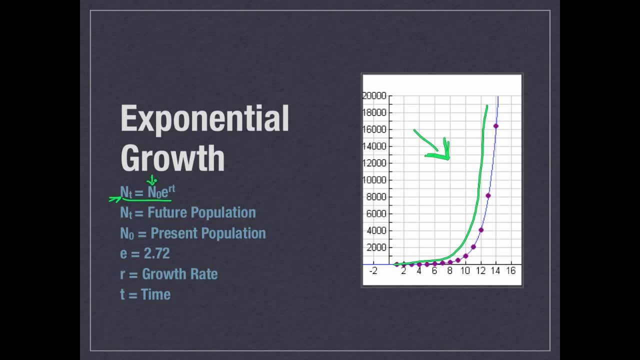 population of a hundred individuals, you would plug 100 in for in sub-zero you have got e, which is the natural logarithm. it's e to the X on your calculator. or you can just plug in 2.72 and that is to the R would be the growth. 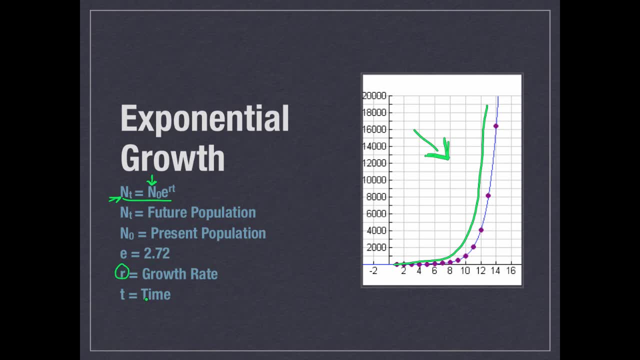 rate. so let's say you've got a growth rate of 2%, that will go in there and time- let's say you've got 12 years, you would plug that in. so I'm not going to run this through an actual calculation, but the way it might look is: in sub T is: 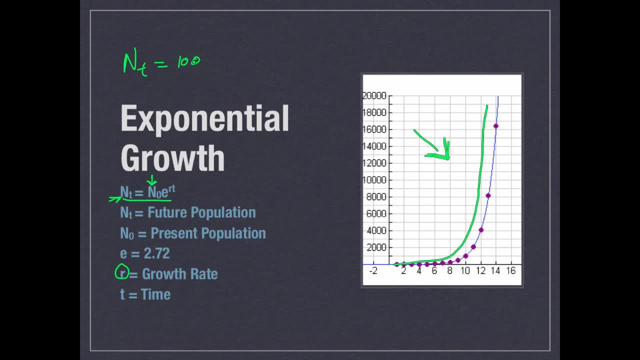 equal to. let's say we have 100 in our original population, and then you're going to multiply that by 2.72 times. let's say our growth rate is- I don't know- 2%, so we're going to put in the 2 and let's say that our time is 2.72, and then you're going to multiply that by 2.72 times. let's say our growth rate is- I don't know, 2%, so we're going to put in the 2 and let's say that our time. 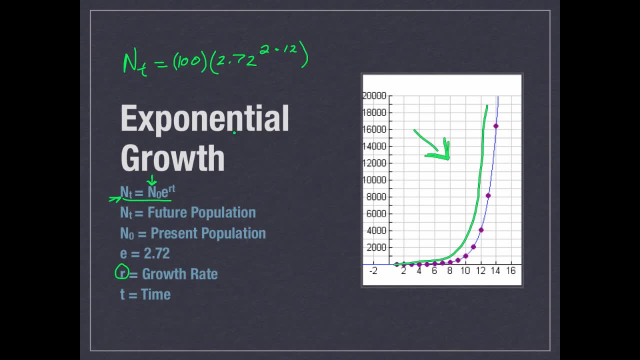 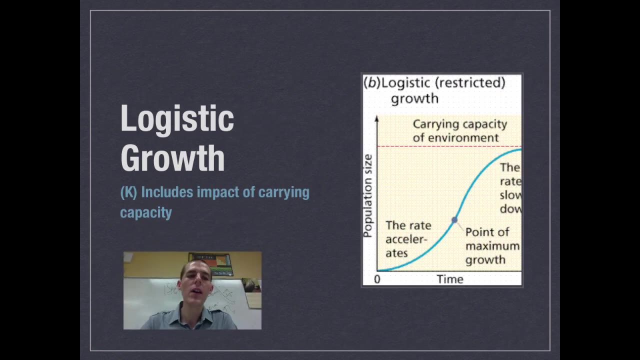 is 12 years. run that through your calculator and it will give you your future population size. so that's something you might see periodically. make sure that you recognize what each one of the terms represents. the other growth model you need to know about is a logistic growth model, and this one is. 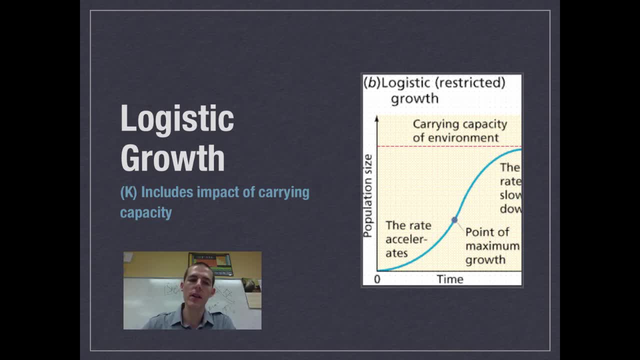 denoted with the capital K, which means that this model is impacted by the carrying capacity of an environment. we talked about carrying capacity in a previous video. carrying capacity is just the maximum number of individuals that the environment can actually support, so there is some limiting factor, whether it 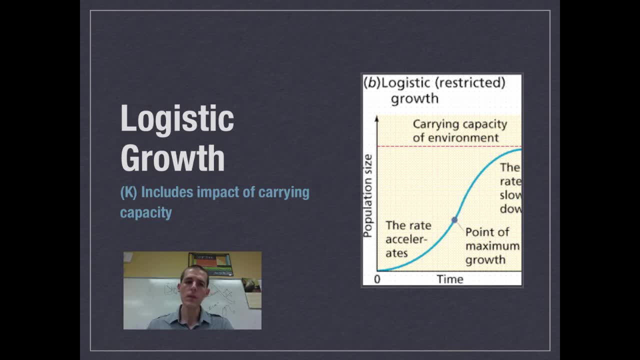 is space or food or predators or whatever. a logistic growth model looks like this. it starts out exponential because there are a few individuals, so they're not really putting pressure on the environment. at this point of maximum growth, which is usually about half of carrying capacity, things start to slow. 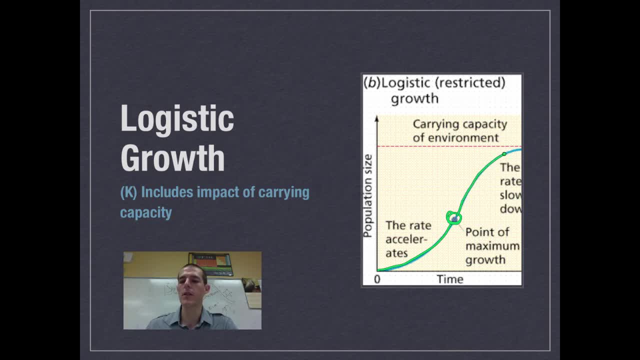 down because your population starts to bump up against the limits of its environment and eventually it will level out and stay pretty flat right around the carrying capacity. so this were an exponential graph, it would continue straight up like this. but due to limits of the environment, the carrying 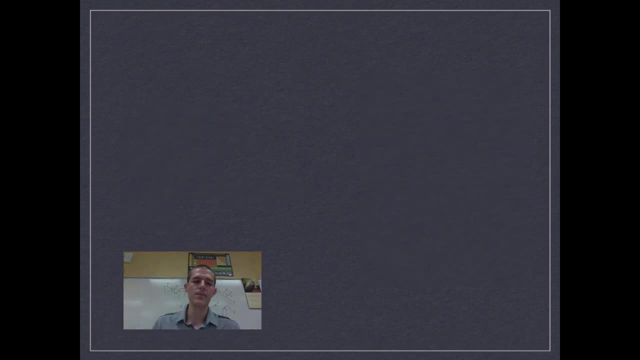 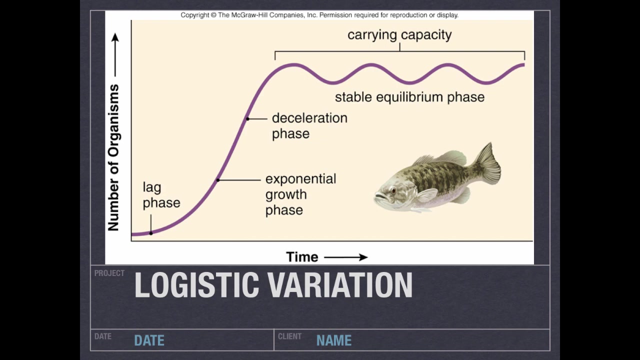 capacity, you get an s-shaped curve, and along with this logistic growth model, there are a couple of variations that you need to know about. one of them is called overshoot and die-off, which is what you see right here, which is basically the idea that most organisms don't hit nice and perfectly. 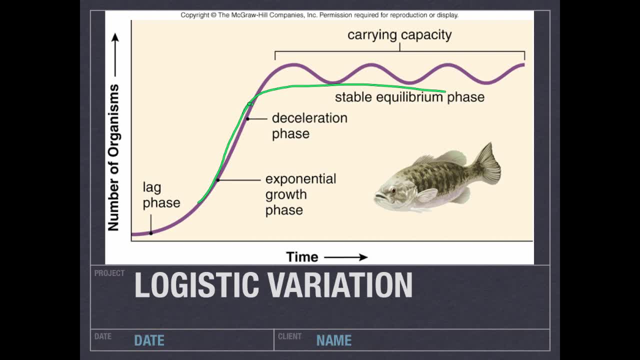 up against that carrying capacity. what they'll do is they will overshoot the carrying capacity, which means there's not enough resources. and since there's not enough resources, they'll die off, and then they'll rebound, and then they'll die off and they'll kind of bounce up and down right around that carrying capacity. it's 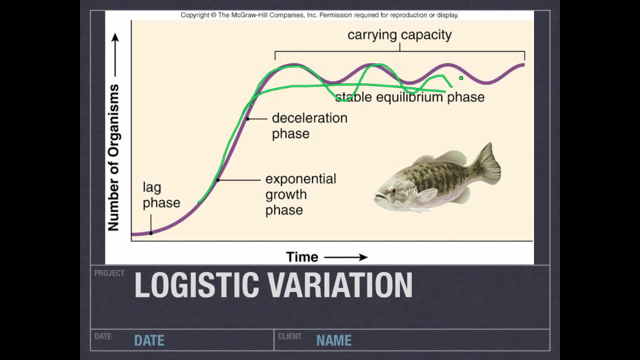 not like they hit the carrying capacity perfectly and just stay there. they'll overshoot it and then die, and then overshoot it and then die. you also see, another variation on the logistic model is predator-prey populations in relation to each other, and the idea behind this is if you've got a population of prey animals, say, the prey. 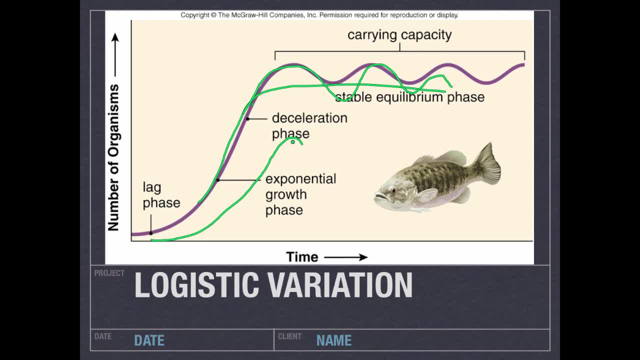 animal population takes off, it grows really fast, and then let's say that we introduce a predator. if there's a lot of prey, that predator is going to become more numerous and more numerous and more numerous, and then suddenly the prey, the predator, will become so numerous that it's going to kill off all of our prey. 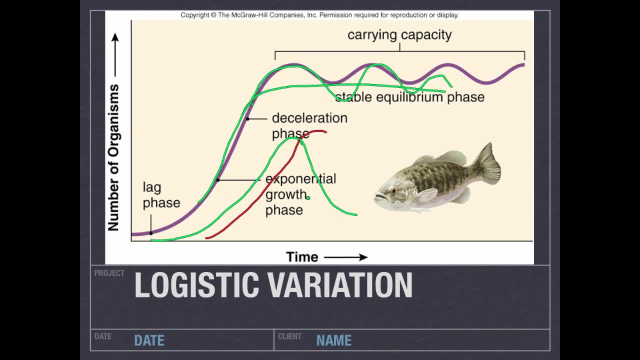 and our prey is going to fall off, and once that prey falls off, there is no food for the predator. so our predator population is going to fall off too, and these two populations are just going to kind of ebb and flow, go up and down with one another, as food is available or not available, whatever the case may be. 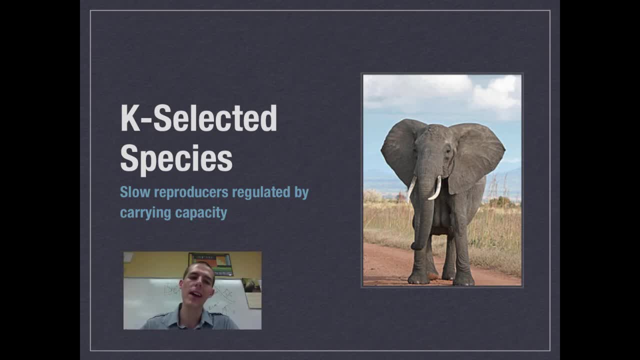 alright, two or three more things to finish up. you need to be aware of case-selected species. case-selected species are species whose populations are dependent on the carrying capacity or carrying capacity of the prey. in the capacity is big letter K, Logistic growth, big letter K. So these are organisms that exhibit. 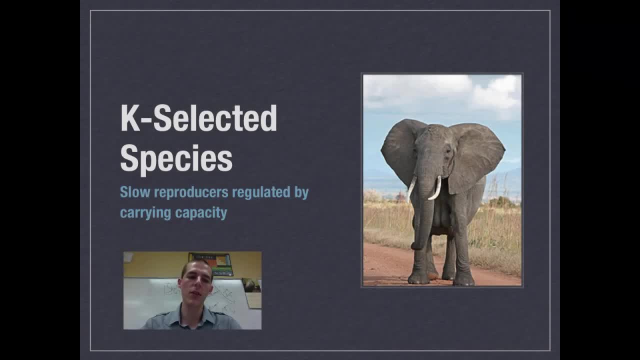 a logistic growth. K-selected species. general characteristics: they are slow reproducers. they're usually large animals, they give lots of care to their young and they don't have many babies at one time. Like I said, their populations are regulated by carrying capacity of an. 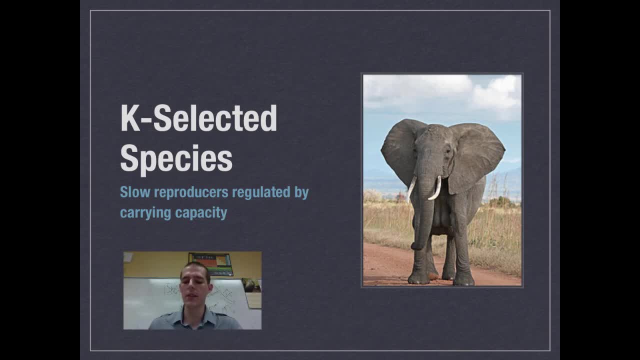 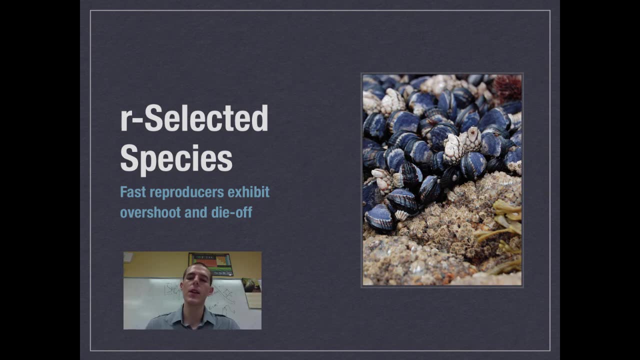 environment. Think of the elephant or humans as a typical K-selected species. Now contrast that with an R-selected species. R-selected is these populations are growing based on the intrinsic growth rate which, if you remember that, was R. so these exhibit exponential growth. They are usually 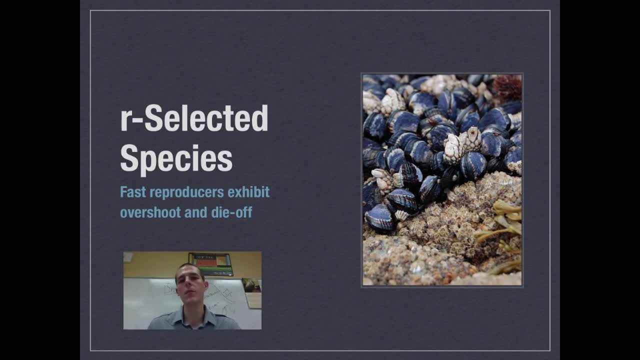 small, they're fast reproducers. they put a ton of babies out there. some survive, some don't, and they generally exhibit, overshoot and die off within their populations. The way I remember this is, R-selected species reproduce like rabbits, And I'm pretty sure too. 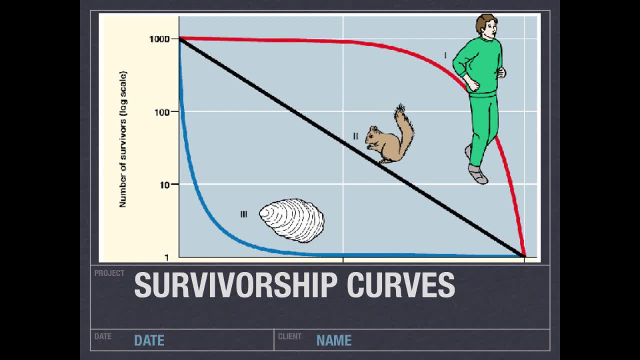 I'm gonna take a few slides and we're done. Using these ideas of carrying capacity- R-selected species, K-selected species- you get a survivorship curve which basically talks about how many individuals in a population make it to the end of the natural lifespan, And you can see. 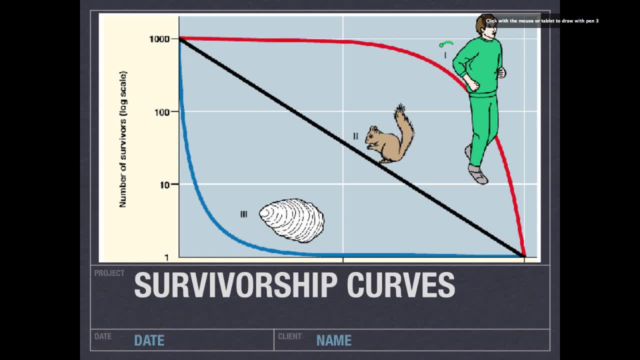 that there are three possibilities here. A type one survivorship curve. These would be your K-selected species. They have a couple babies, they take good care of those babies, those babies live for a long time and then down towards the end of the life there's. 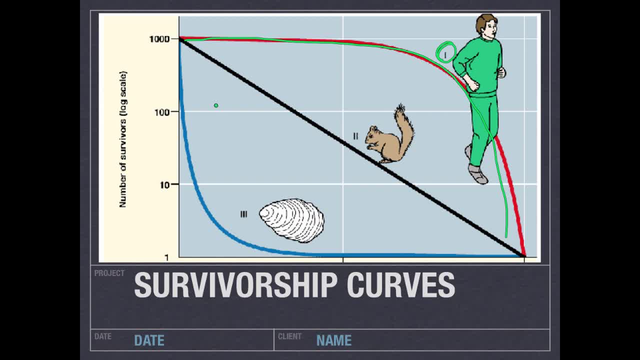 a pretty quick die off. The exact opposite of this would be your R-selected species. They have a ton of babies. most of those babies die off very early in life and then the remainders survive out the rest of their days, And then in between you've got most everything else and they show a pretty even die off over. 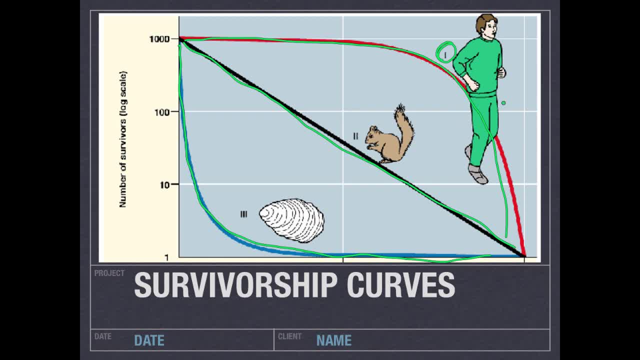 time. So type one: survivorship curve: lots of babies live and then most die off at the end of their years. Type three survivorship: tons of babies that die and then a couple live and then type two is in between the two of those. 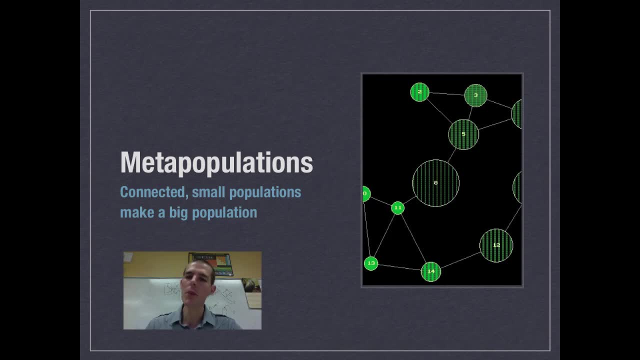 And we're going to wrap up with the idea of metapopulations. Metapopulations is basically talking about populations that are connected to one another. So let's say we've got a ton of mountain ranges. In these mountain ranges live cougars, mountain lions, All those cougar.